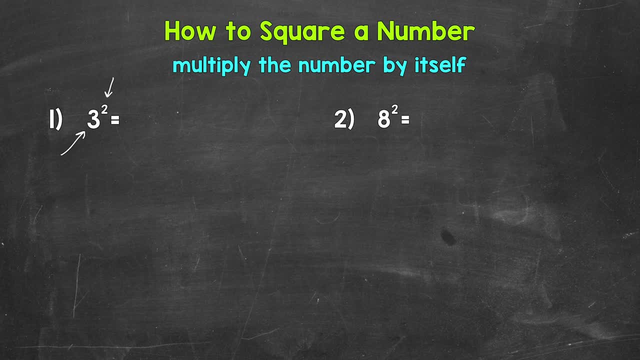 The exponent tells us how many times to expand the base out and multiply. Let me rewrite this here: So 3 squared equals well, this means 3 times 3. 3. 3. 3. 3. 3.. 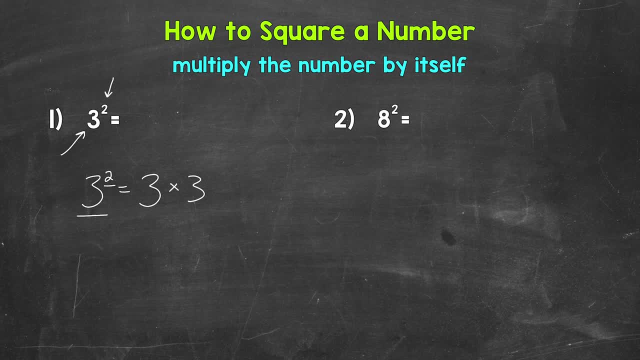 3. The base of 3 expanded out 2 times. So we are multiplying that number by itself 3 times 3.. And we know that 3 times 3 equals 9.. 3 squared equals 9. And it's as simple as that. 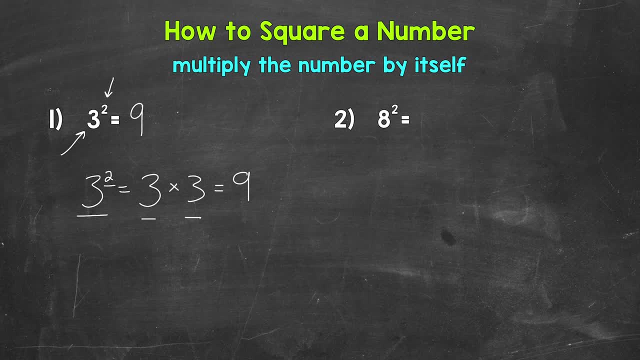 Now, a common mistake would be to do 3 times 2.. Don't multiply the base by the exponent. That would give us 6. Which is incorrect. Remember, expand the base out however many times the exponent tells you. Before I move on to number 2, I do want to mention why we call it squaring a number. 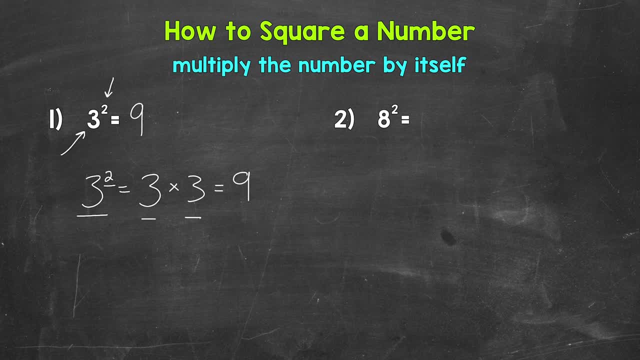 If we take a look at a square, we can see why we call it squaring a number. For example, if we have a square with side lengths of 3, we can find the area of that square by doing 3 squares, Or 3 times 3.. 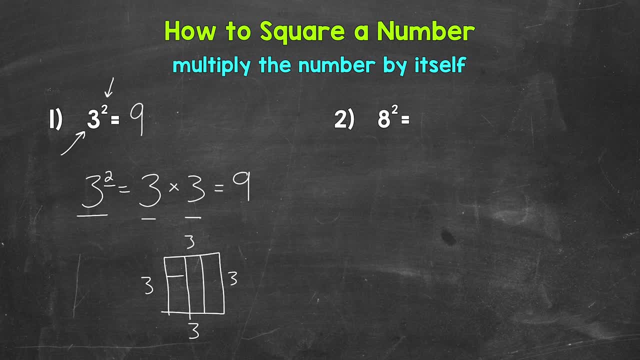 So 3 by 3. That gives us an area of 9.. We can square a side length to find the area of a square. So you can see the relationship between squaring a number and the area of a square. Let's move on to number 2, where we have 8 squared. 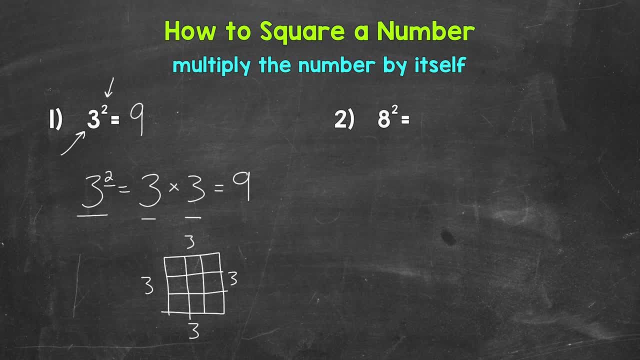 Now, 8 squared, that means 8 times 2.. 8 times 8.. So 8 squared equals 8 times 8.. The base of 8 expanded out 2 times 8 times 8 equals 64.. 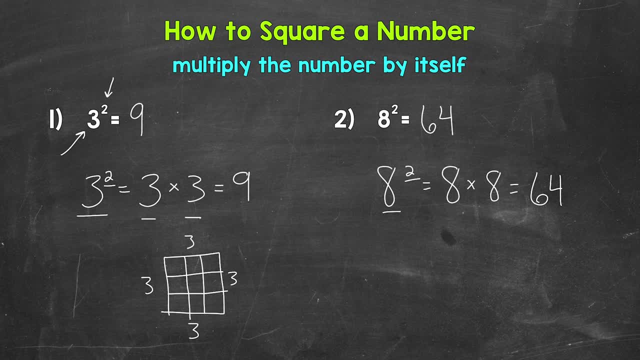 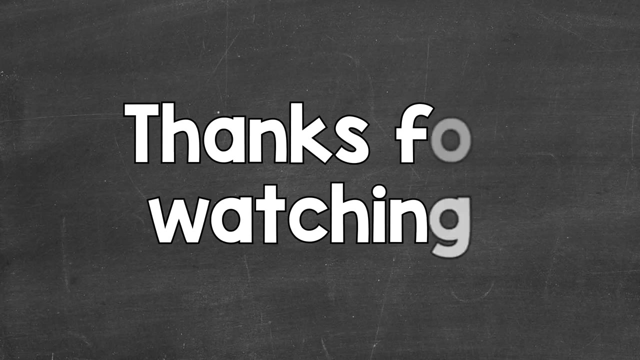 So 8 squared equals 64.. So there you have it. There's how to square a number. Multiply the number by itself. You're expanding that number out twice and multiplying. I hope that helped. Thanks so much for watching. Until next time, peace.